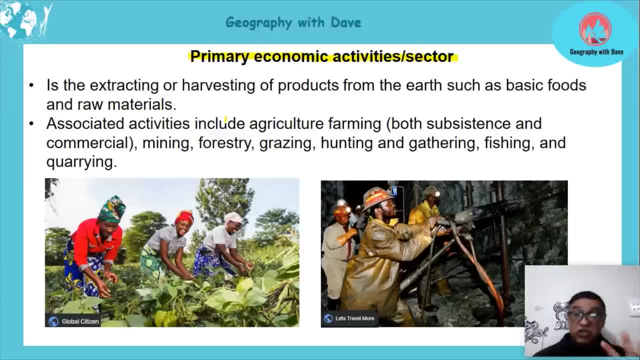 all right in your other grades and whatever. Okay, but it's good we do it first And it's important we do it first And it's important we do it first And it's important we do it first. We do the sectors first because later on in economic geography we're going to take each 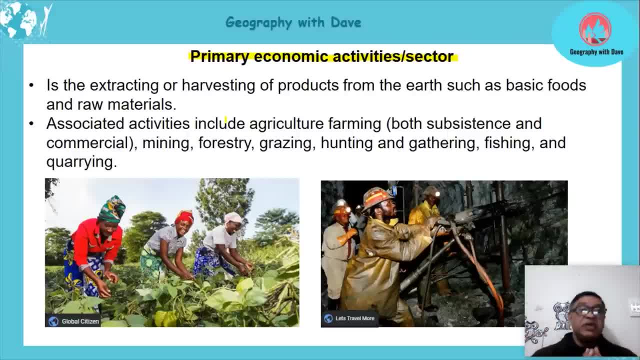 sector and explore it to great depth. Okay, so let's start. So we said primary sector is the extracting or harvesting of products from the earth, such as your basic foods, your vegetables, et cetera. You understand, And your raw materials all right, like your gold. 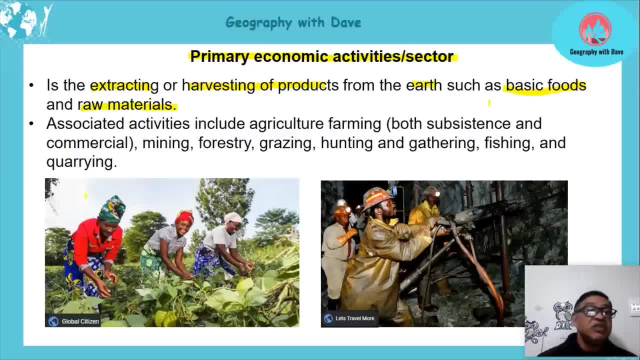 your iron ore, et cetera. So you can see, here these ladies are happy because they're producing quality food there. Can you see it? All right, your basic foods. And these strongmen here like me, all right, are busy mining and extracting raw materials such as gold and iron ore, et cetera. 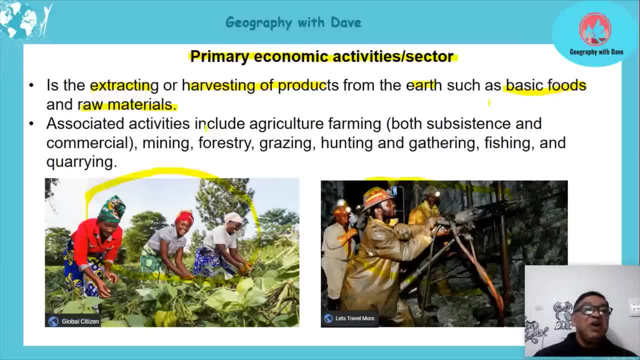 Okay, so we know it includes various things: Agricultural farming, both subsistence and commercial. It includes mining, forestry, grazing for cattle et cetera, hunting, gathering, fishing, quarrying, where you dynamite the area to get your gravel, et cetera. 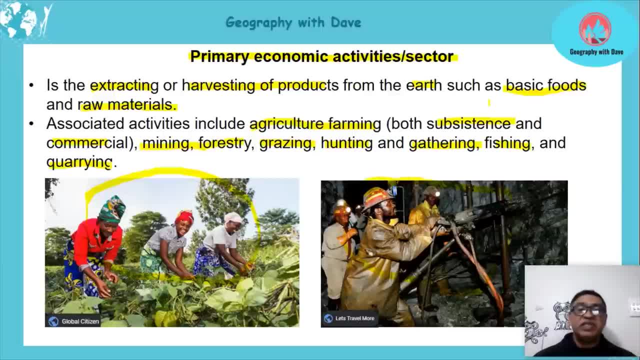 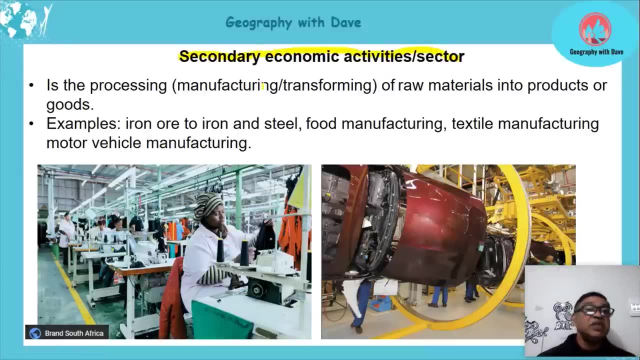 These are some of the many examples, that of primary economic activity or sector. Okay then, let's go on, learners. Let's look at the secondary economic activity or sector, And this involves processing. other words could be manufacturing, transforming of raw materials. 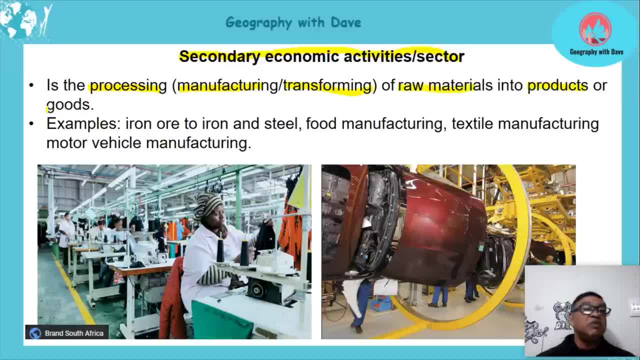 into products, or sometime known as your goods. all right, That's more valuable. I do apologize some of the time, but I do apologize sometimes. but I do apologize sometimes, but I do apologize. my face may just stop moving. all right, my internet is not the best today, okay, so don't laugh at me. 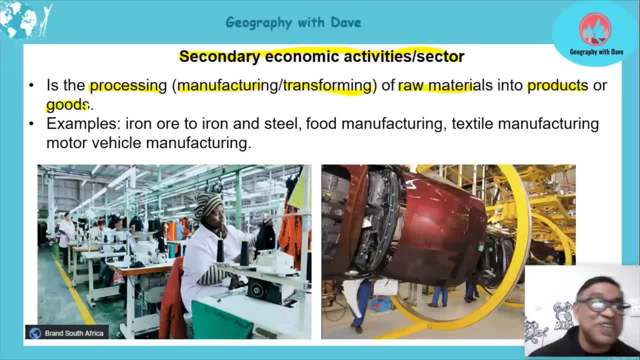 when i look funny and my face stops moving and my hands stop moving. okay, let's get back. so it's products. goods like, for instance: yeah, learners, you can take iron ore and produce iron and steel. many of us won't just take the iron and steel and drive around. okay, so it's a product that's. 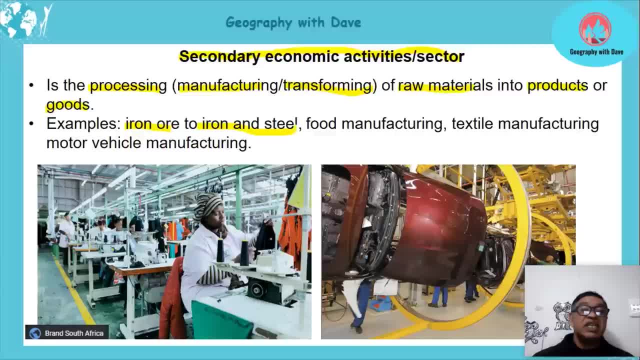 produced and we can have Finnish goods when we take that iron and steel and use it to make a car. well, i hope our cars got iron and steel, because sometimes when you kneel against the car it bends okay. so i hope it has iron and steel in it, right. so that's one of the things, and, of course, 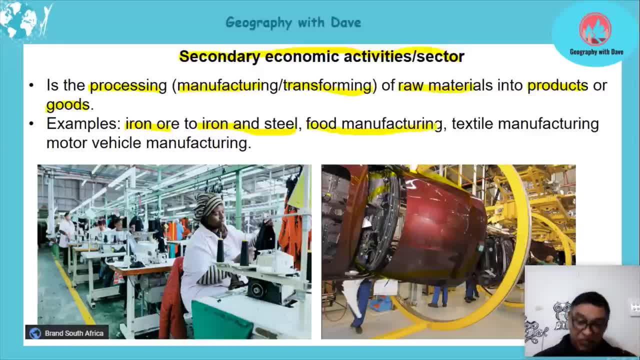 food manufacturing. all right, we finish. product is your food. you get your breakfast cereals, you eat it. your textiles- you understand. and, of course, another Finnish product, your motor vehicle. down here, what you can use in terms of motor vehicle manufacturing, all right, can you see there? there's this lady here, uh, doing textile manufacturing clothes. 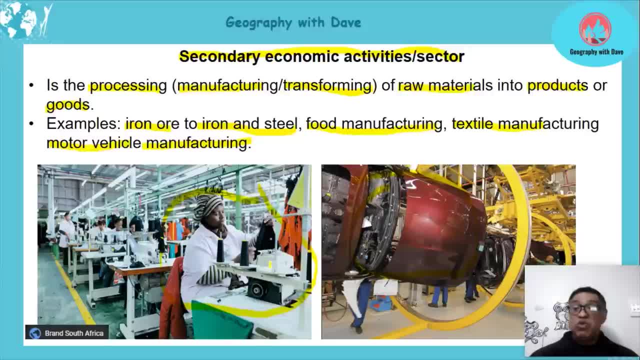 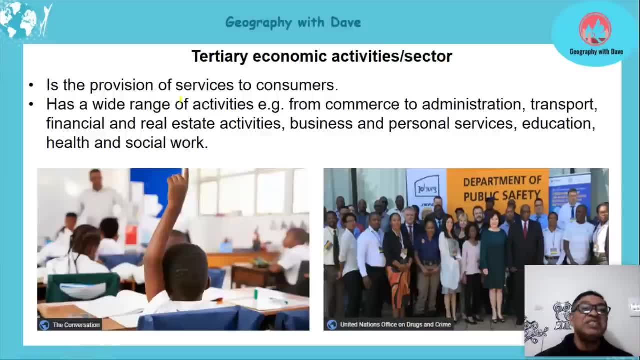 i i admire. i'm very scared to go near sewing machine. i may sew my hands up, okay, but that's the idea of secondary economic activities. and then we have tertiary economic activities, or sector all right, and this main thing is services to the consumers. all right, people. 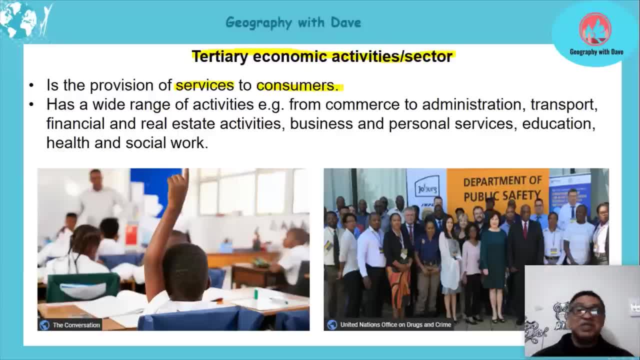 like different services, so it's to the consumers who want that service. so it's a wide range. this is really wide range of activities. all right, we, for instance, we have commerce, your administration, people handling your accounts and whatever, transport. all right, financial, the money, the banks, the big boys. all right, real estate activities. 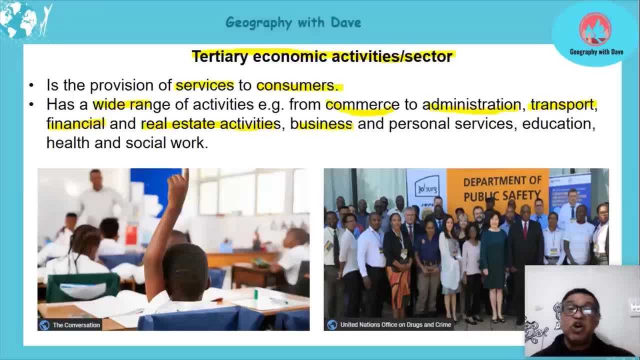 selling of houses, your general businesses, your shops, etc. your personal services, education, all right, like this place here at the school. okay, i wish all of you- i hope all of you are like this young man. eh, got his hand up immediately. i'm sure you're all with me today. all right, you're doing this. 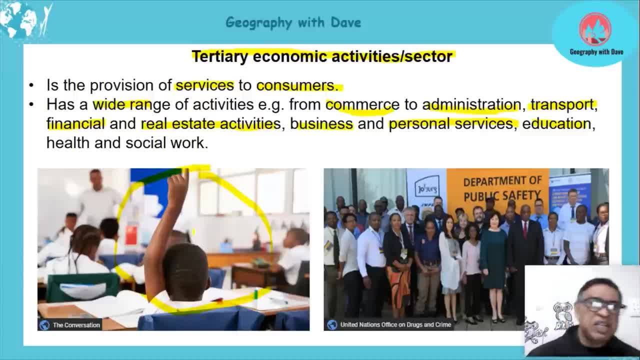 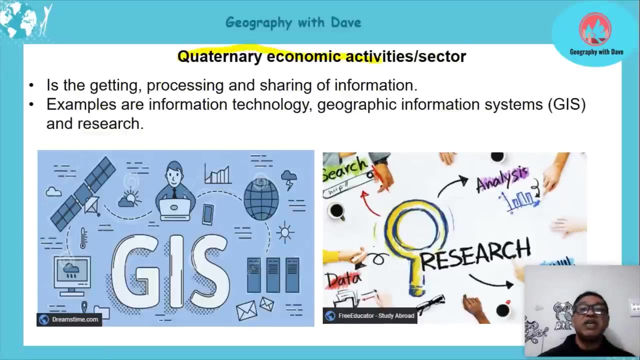 all are geographers, so you'll always be smart and know the answers. okay, so we have all that health social worker, all services like this department of public health safety, rather, is a service being offered? okay, right, and let's get on, and we look at quaternary economic activities or sectors. 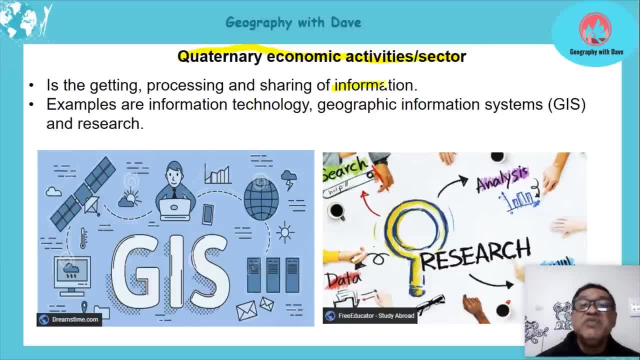 this deals with information. your main word is information. yeah, it'll involve the getting of the information, or gathering of the information. that gis does with remote sensing and whatever. all right, it's processing of the information. gis is a perfect example of the same. you process it. 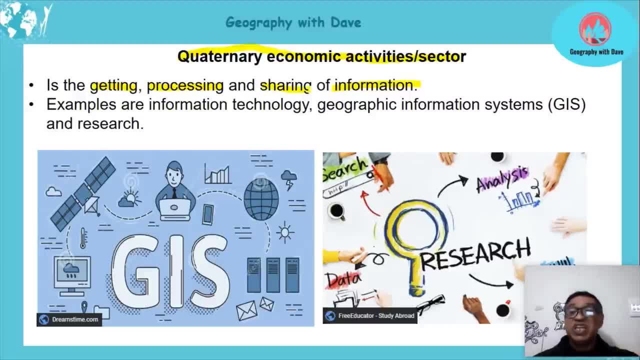 and then you share, like in data sharing, you're sharing the information, all right, so it involves many things. all right, there's your gis here, okay, and there you can see research, where you're getting your information from the people. all right, primary data, etc. you're picking up, can. 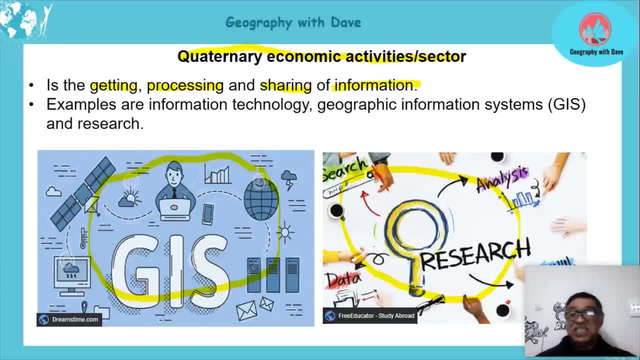 you see other sections are related. all right, you're getting the stuff okay through research, so it'll involve things like information technology, geographic information systems and your general research. some of the examples of your quaternary: it's still, in terms of the other ones, moran, but it's growing. 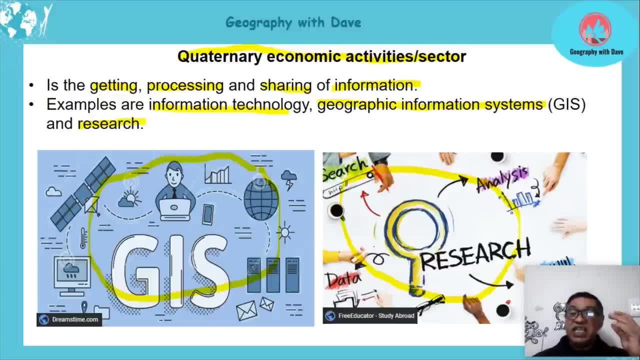 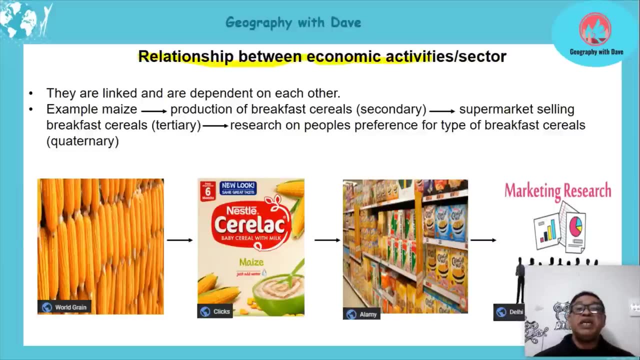 remember, at one stage, with this primary, tertiary, and primary, secondary and tertiary, now quaternary is a sector on its own and growing. okay, right, let's go on. so the now we look at the relationship between the economic activities and sectors. all right, uh, actually they are linked, learners linked, and are dependent on each other. also, okay, now let's look at why. 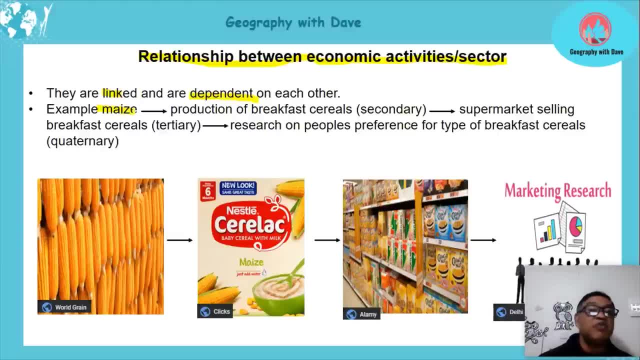 the maze is far, of course, that's your primary. okay, the production of breakfast cereals? there's the maze here. all right, the production of breakfast cereals is your secondary activity, all right, or yes, comic activity activity. the supermarket selling the breakfast serials is your tertiary. 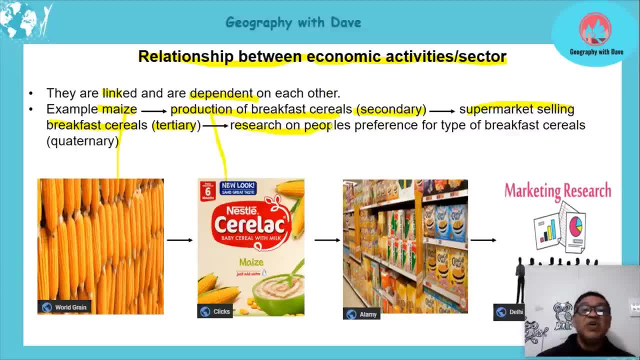 all right, can you see the flow here? all right, then. research on people's preferences for type of breakfast cereals. is your what, nary? okay, so each one. in fact, the research is also important, because what will happen here is: let's take this down here, all right. 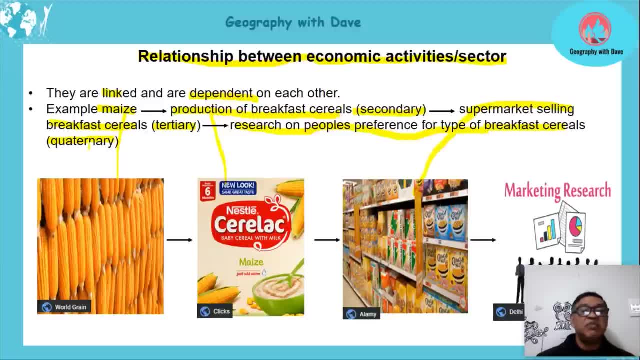 the shop selling it, all right, and your research are making a big mess of it here down here. so let's take an example. let's say research shows, all right, that there's a huge buying of this product, you understand, of this breakfast cereal from from your maze. okay, huge buying of it. so what happens? 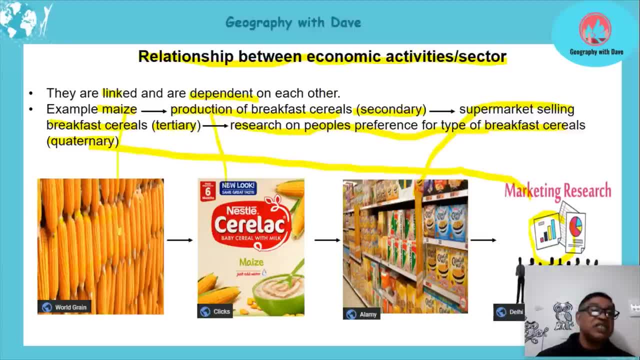 now there's an increase in production here, which will have more raw materials. more cereals will produce, more will be placed in the shop to be sold. if it decreases in terms of demand, the opposite will happen. can you see how linked they are? like how i did my little lines running everywhere down. 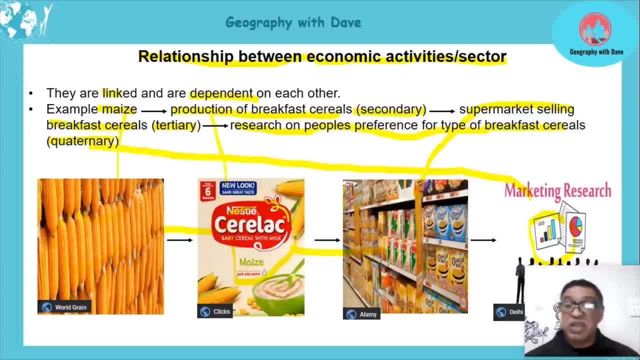 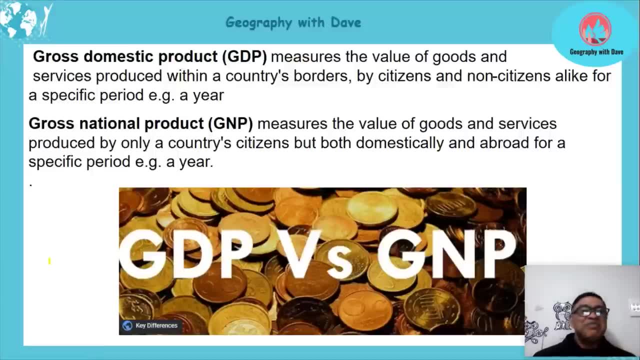 here. okay, i hope you have your breakfast cereals every morning, like i don't. i'm sorry, i do. okay, but now we're going to look at the value of contribution, okay, of of these sectors in terms of development etc. but please note, i know the curriculum doesn't state define gnp or gdp etc. 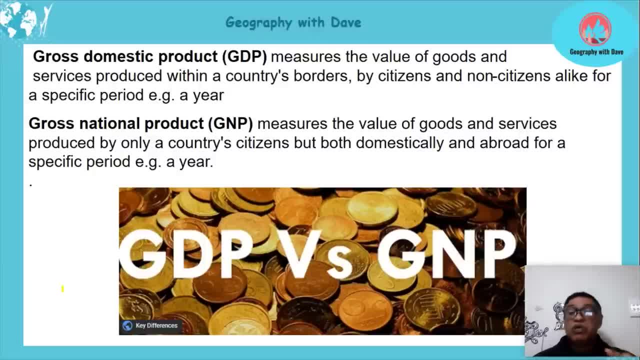 but it's important. i know you've done it before, but it's important to revise your concepts, learners, because if you don't understand your concept and it's a applied in an explanation, you're going to have problems understanding the explanation. so let's look at these concepts first before we go further. all right, let's look at the first one: gross. 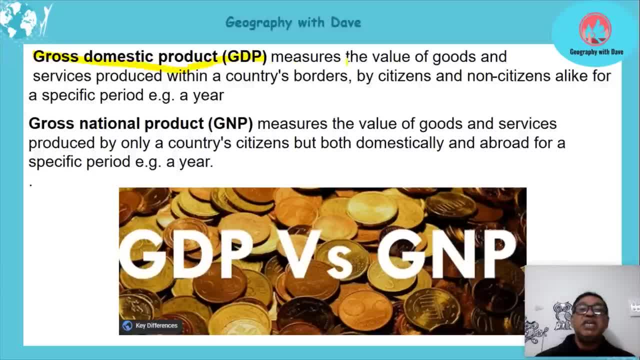 domestic product. what is it? it measures the value of goods and services produced within a country's borders. all right, all the production like in south africa, within south africa. all right, and by citizens and non-citizens alike. whoever is in south africa and they producing, okay, whether it's citizens. 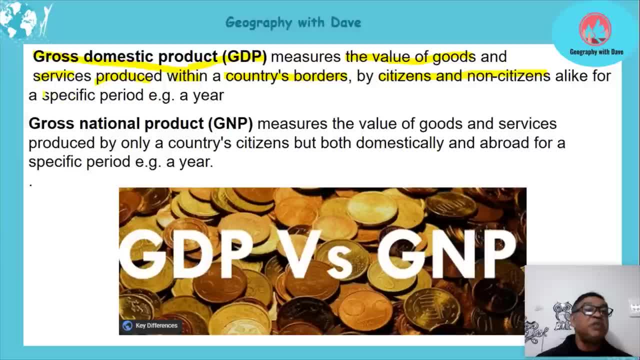 non-citizens, all right, and it's for a specific period, generally a year. that's how it's worked out. all right, let's look at gross national product again, the value of goods and services produced only by a country's citizens. now this is no more non-citizens, but it also includes domestically and abroad means within the 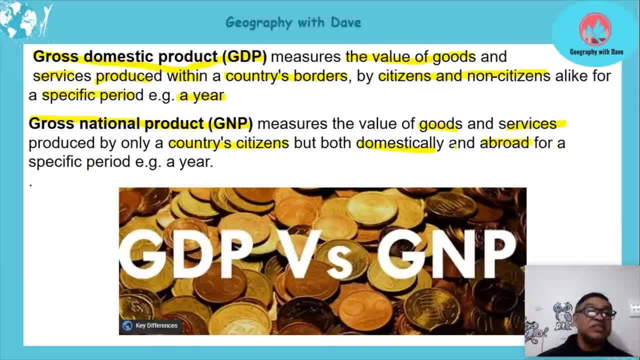 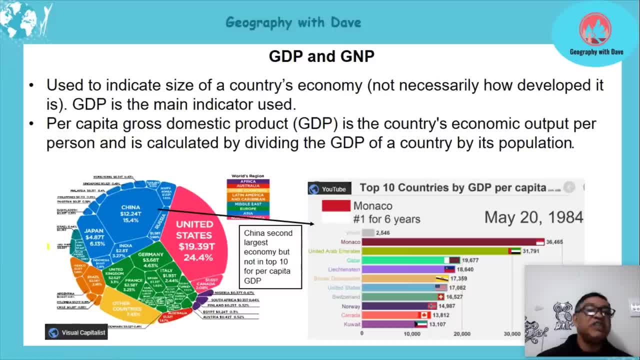 understanding of this. all right, we've got an understanding of this. all right, let me go further if it allows me. let me go further if it allows me. now. let's look at this- the gdp and the gnp- and look at how it works. all right, it's used to indicate the size of a country's economy. 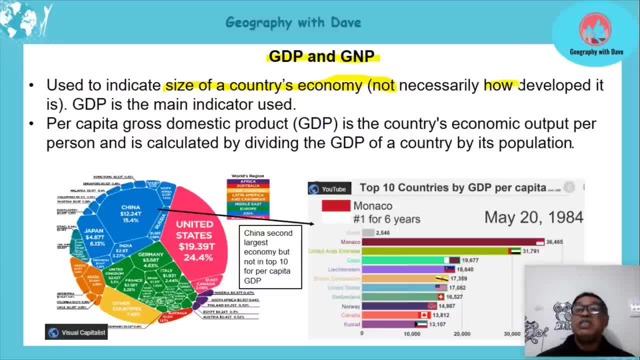 and not necessarily how developed it is. okay, i'm gonna come to that point now, because i know you're thinking: what am i saying here? all right, let's take it step by step, all right? the gdp, obviously, is the main indicator used to determine the size of a country's economy. 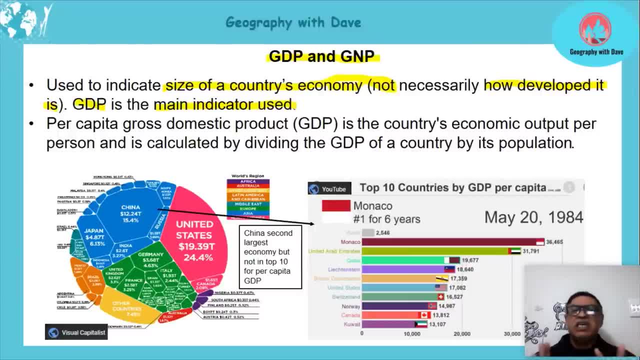 now i'm gonna throw in another concept into the mix in order to explain this size and and the difference between size and how developed a country is. i'm not throwing this- i know it's not in your curriculum, but it will make the understanding easier. okay, i'm going to. concept of per capita gross domestic product. all right, just domestic product. 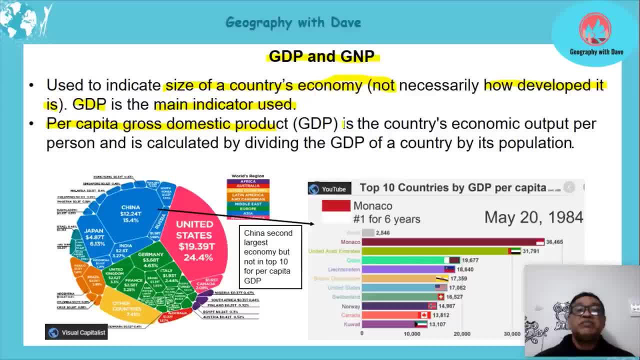 referring to gdp. okay, right, is the country's economic output per person. now, how do we work this out? which is how we calculate it. we divide the overall gdp, or the goods and services within the boundaries of a country. blah, blah, blah. you've got that all right by its. 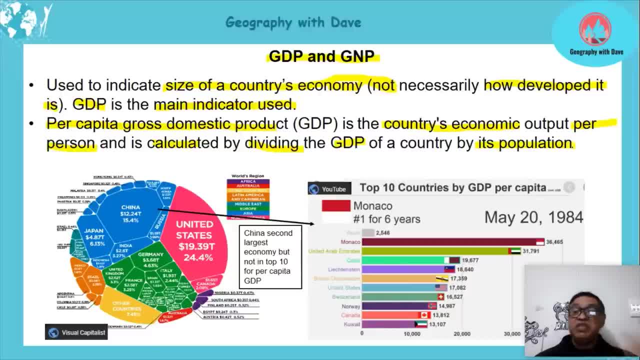 population. so let's say a country's gdp is one trillion dollars and it has 50 million people. we then divided the 1 trillion by the 50 million to get an average per person. so obviously, if there's higher development, the average would be higher. okay, you got that. now let's look at what we meant. 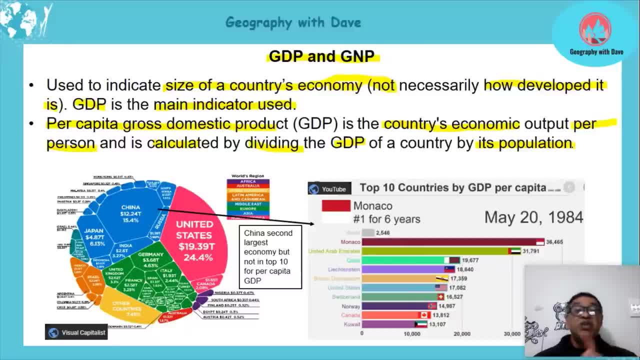 by. it talks about the size of the economy and not how developed it is. all right, let's look at china. you're huge, second largest economy in the world after the united states. all right, but look at the top 10 countries. gdp per capita: it doesn't even appear here. 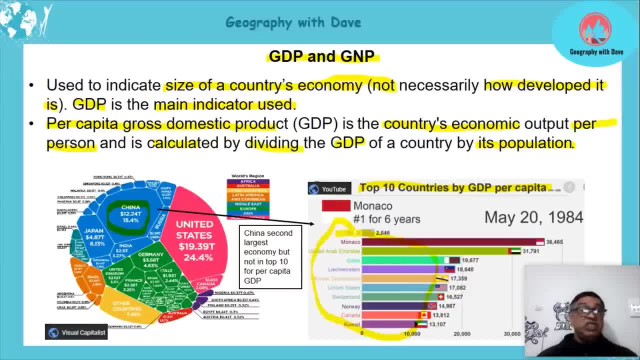 okay. so it may have a large economy because it has a lot of people, you understand, uh, over 1.3, 1.4 billion people or more, and counting, you understand. but although it produces so much, if you divide what the gdp of china is, you understand, of 12.24 trillion dollars, and you divide it by uh, 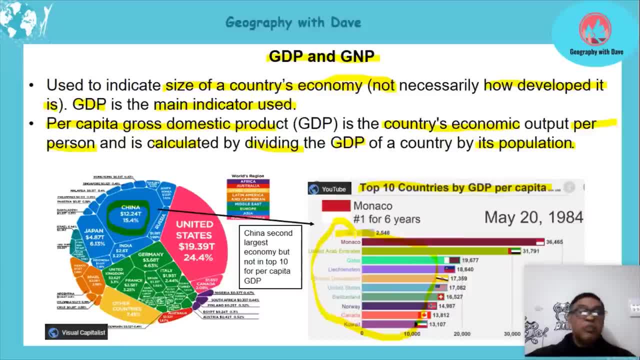 over 1.4 billion people or more, approximately more. you understand, you'll find that the per capita gross domestic product is lower than maybe if you take monaco, which has maybe a certain number of people, has a lower, uh, number of, uh, sorry, has a lower population, and if you divide it it's different. 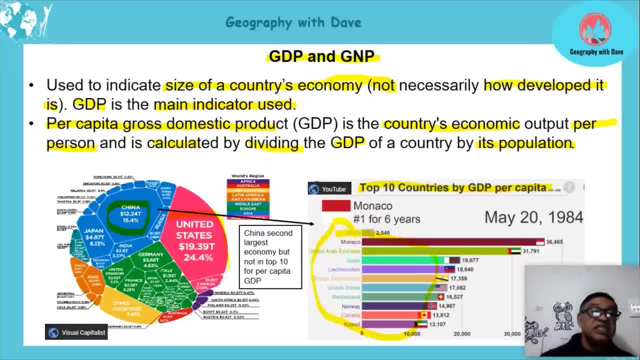 i've got another example here: you take the united states right and it makes 19.39 million billion. okay, or, for instance, let's take- let's take something like japan, which is better example: 4.87 trillion people, uh, trillion in terms of gdp dollars. all right, i do. 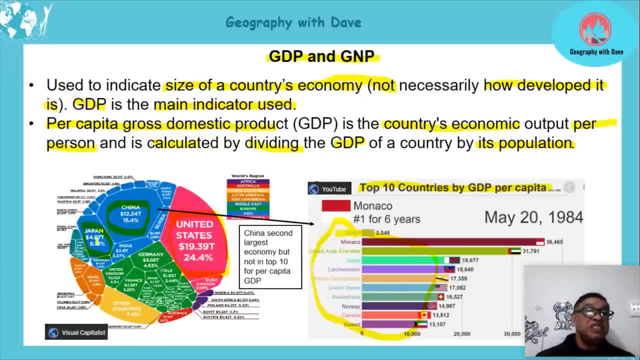 apologize for that. so it's much smaller in terms of the gdp, you understand, but china has 1.4 billion people compared to japan, which may have 100 or so million people, and if you divide you'll find that that the capita gdp for japan is greater. all right, you've got that, let's go on. 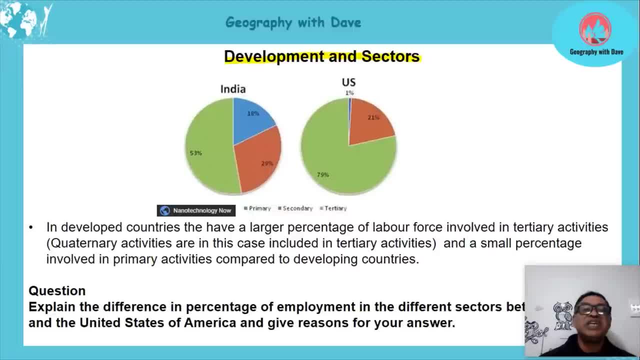 now let's look at development and how the sectors indicate development. all right. now let's look at it down here. let's look at ufc, say- and during this period of course it changes all the time- and india: in usa, at this stage, the tertiary employment right was 79 percent, all right, whereas in india employment in tertiary was 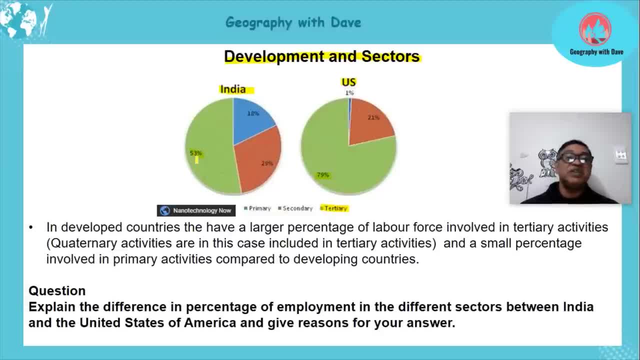 53, huge difference, all right. and if you look at india, the primary was 18 and the usa it was one percent. all right. now that is a good indication that in developed countries they- they, not they- have a larger percentage of labor force involved in tertiary activities and quaternaries activities included in tertiary. 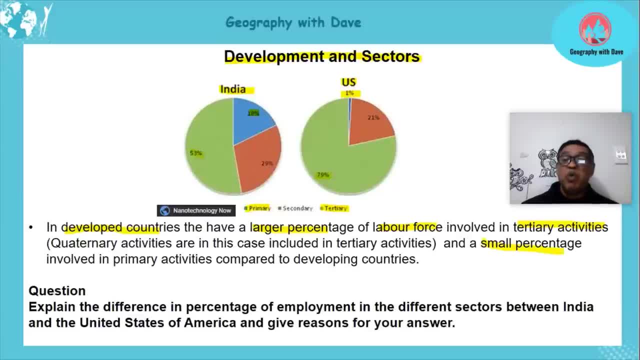 in this little resource, all right, and a small percentage involved in primary activities compared to developing countries, all right. now we have these highly industrialized because of the large population of india and maybe the industries would be more than us. sometimes you would find that trend that industries are higher and developed, but not necessarily. that is why i use 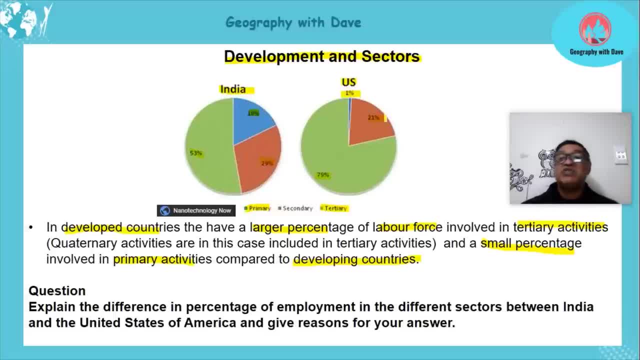 this example. all right to clarify that, that you can have situations different. but the biggest indicator here is looking at the tertiary and primary and the labor force or employment in those sectors actually gives you a lovely indication of the development. all right, i just threw a question here. learners explain the difference in percentage of employment. 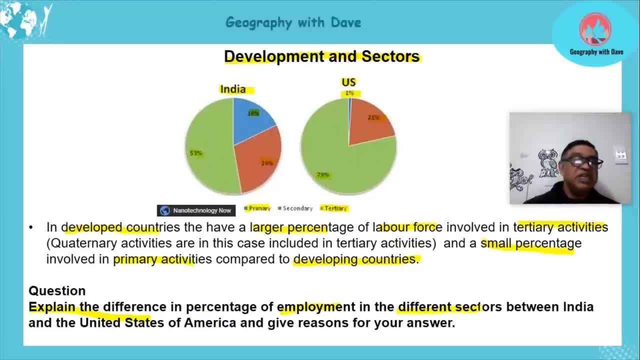 between different sectors, uh, between india and the united states, and we just discussed that. can you see i'm phrasing it in the question that tertiary in the united states is higher compared to india, whereas in india the employment is higher for primary compared to the united states. all right, and uh give reasons for your answer. we can then talk about. 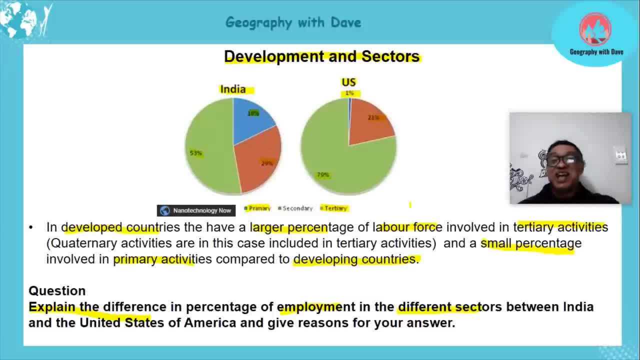 how developed the country is. all right. united states is highly developed compared to india- all right, they have all the resources, etc. therefore, people's per capita income is higher. more machinery is used in the in the united states compared to a developing country where there's still a subsistence economy. there's so many things that you can. 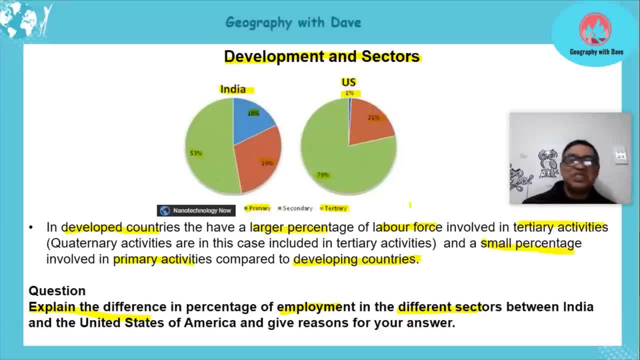 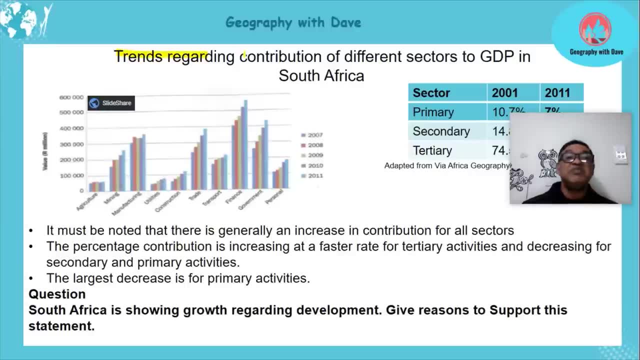 talk about in this question. just through you, a little question there. all right, let's go on trends regarding contribution of different sectors to gdp in south africa. let's look at south africa, all right. uh, i want to look at two little things here. number one: there's a little information here showing you from 2001. 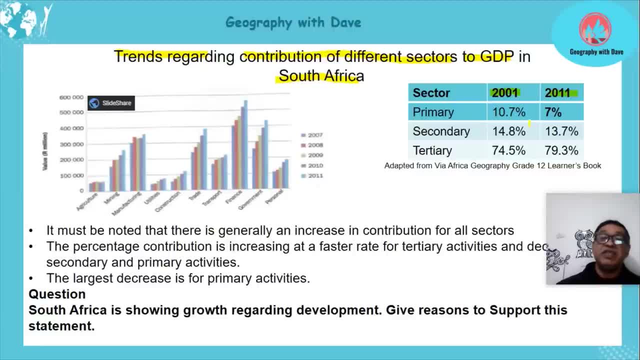 uh to 2011 and what we noticed? that in the primary sector it dropped from 10.7 to 7 percent. there's a drop in the secondary sector. it dropped from 14 to 13.7 and in the tertiary sector it increased from 74.5 to 79. all right. 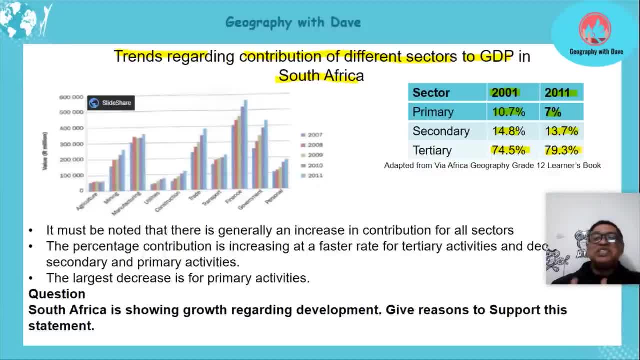 which shows that there's growth in south africa regarding moving towards more development. all right that. and now more machinery is being used in the primary sector as better quality of life- all right, although we still have various challenges. okay, but it's moving forward, all right. therefore, the tertiary sector is actually increasing: better education, more money, more. 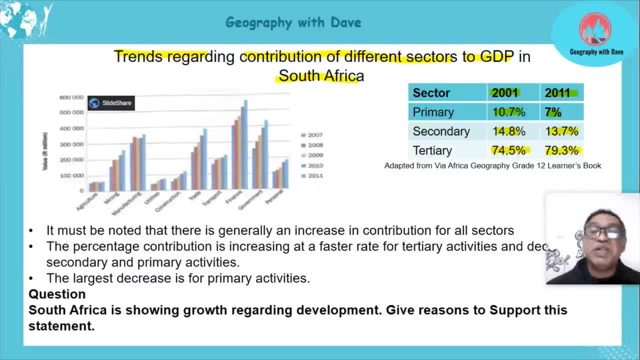 finances available to too many people. all right. so we are moving in the right or in the growth position regarding development, all right. so you must notice here, all right, that when we looked at this, we saw that there's growth happening. now, how is the growth happening? if you look here, you find this general growth. this is agriculture, which is 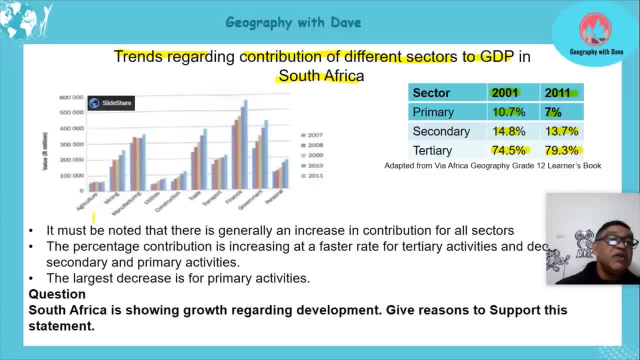 primary mining, which is primary right in this area. here, that's your primary. then we have secondary, okay, and then, of course, from there to there, okay, secondary. then we have our tertiary right sectors and we notice that growth is generally occurring as the years go by, you understand, from 2007 to 2011. 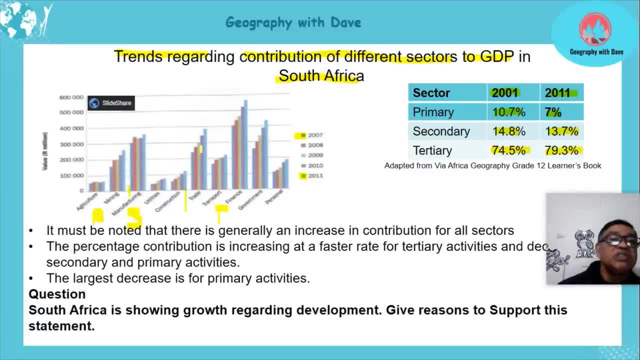 all right. growth is happening in more or less all sectors in this area. can you see it? in all sectors growth is happening. okay, but what would you notice? that if you look at this agriculture all right and sometimes at mining, and we compare it here, you'll notice that generally growth is happening faster in the 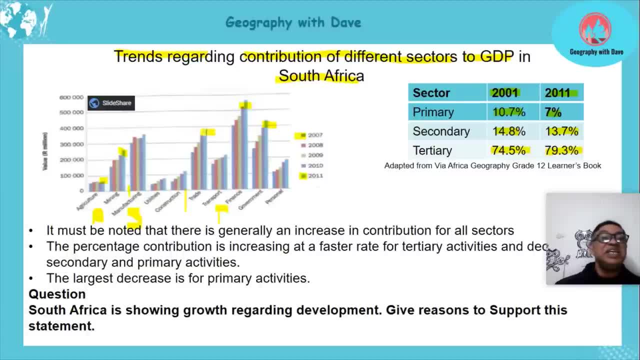 tertiary and generally the tertiary. there it's happening much faster than the other sectors, which is showing you all right development happening in south africa. we've become more and more developed, as it is all right. we're not there yet, but we're becoming more all right. so what can we see from this? 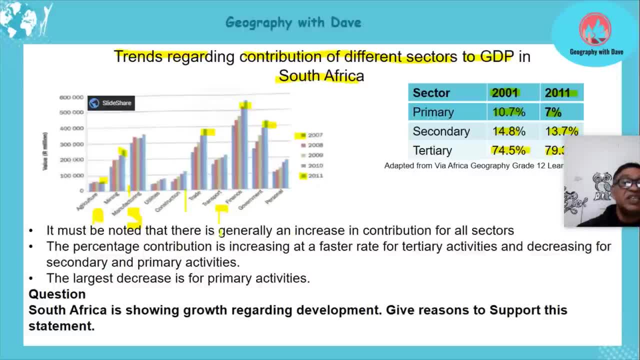 that it must be noted that there's a general increase in contribution from all sectors- all right, but the percentage contribution is increasing at a faster rate for tertiary activities- all right- and decreasing for secondary activities. please note that learners- each one is increasing, but this is happening because the tertiary activity percentage is. 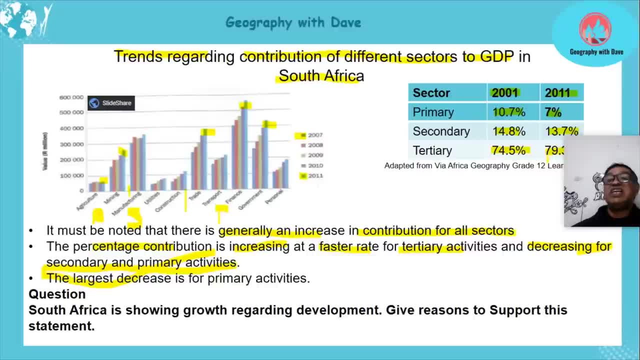 increasing at a much faster rate. have you got that? learners? all right, so we can look at this question. just a little thing. it's all the same information. so I was showing growth regarding development. give reasons for your to support this statement. all right, and you can see here. all right, there's. 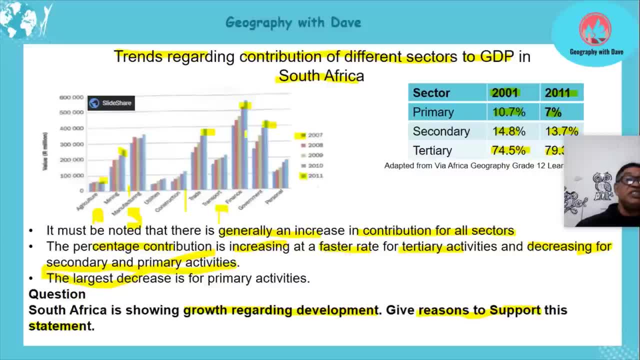 growth happening right through. all right, it's increasing continuously from all sectors, and the tertiary sector is increasing much faster than the other sectors. all right, just based on this. there will be various other answers that you could look at here, and, of course, you have to base it on. 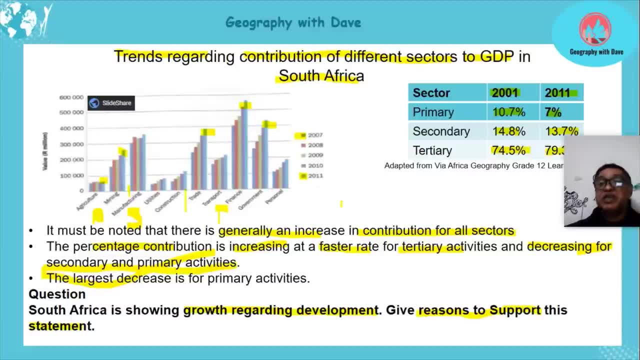 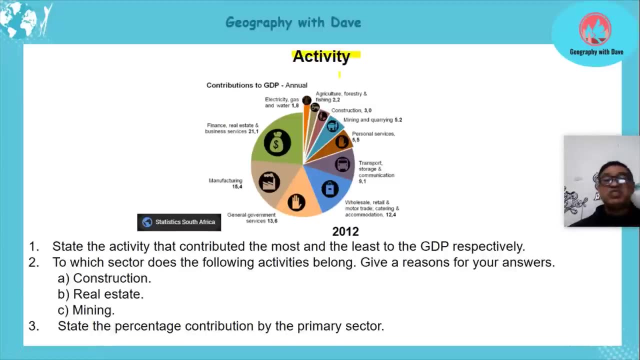 the resource that's given to you in your assessment. okay, if you ask for general answers, you can go generally. okay, so some interesting Trends. okay, in terms of South Africa, I just got a little activity here and, please, you must learn. don't assume it's simple. learn how to interpret your resources, your 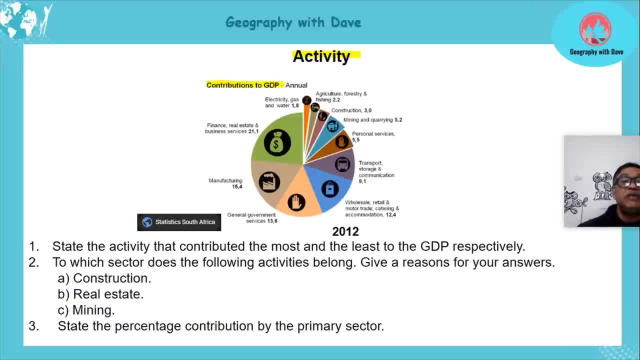 tables. okay, this shows contribution to GDP right by various activities. they can be grouped into primary, secondary and tertiary, all right. so first question: state the activity that contributed the most to the GDP, at least respectively. so I look at my figures- these are my uh percentages, all right, and I'm looking here. I see 12.4, 9.5, 5.5.2, 3.0, 2.2, 1.8 and I see 1.8 is the lowest. I didn't. 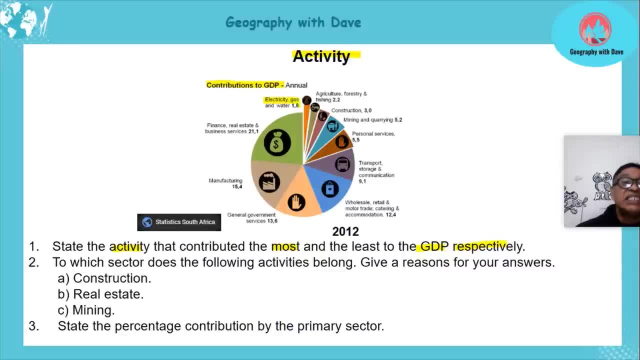 ask you for an economic. all right, so it's electricity and gas which is the lowest, the least. okay, then I go for the most and I keep checking 12.4. uh, nine point one, four, six, seven, eight, nine and a half five, six, 109, fifty twenty five, thirty nine, fifty. 'm last one. i see you cash balance check. the hasn't asked you for the spoiled components here in country, which is the lowest, the lowest, and have stating that the last economic like you see, the lowest. i have seen you, Colin robin. you have seen you committees, cái las seen minors by the law of u l t. yeah, i will see twenties致 sagen per se and people itas e ones that i'm Kr 89. okay, it's so. it's that the lowest, 황 팔 u Group gave the lowest. so working for the ikr ii b. 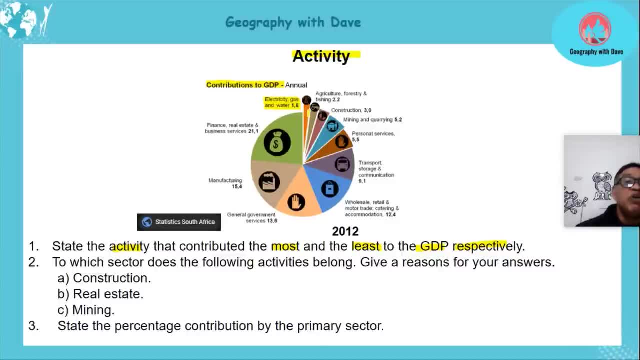 9.1, 5.1, 5.23, 2.2 and i'm going on. you understand and i'm seeing there's nothing more than 21 and i hope to be corrected. yes, i am, and that is your finance and real estate and business services. 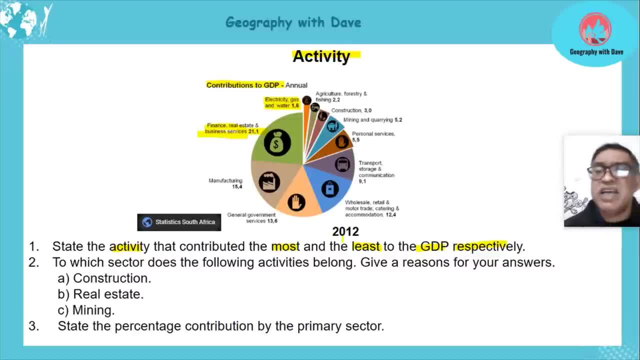 that contribute to the most. can you see it? uh, lannis, you get questions like this on various occasions and sometimes he's just taking the information from there. okay, right now let's look at the next question, which takes it a little further. which sector does the following activities belong? all right, and give reasons for your answers. all right, let's take. 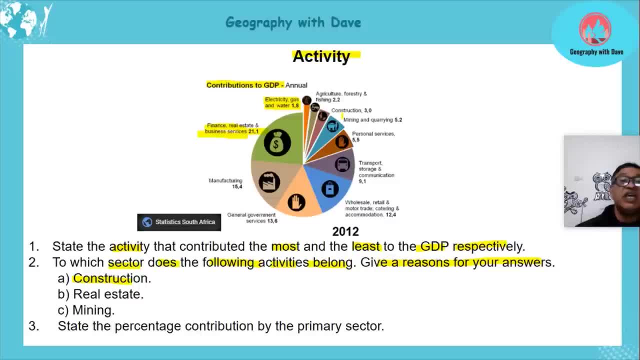 construction, all right, construction there. it is there. you're constructing, you're making something. if you construct it, it's a secondary activity. all right, you're constructing something. all right then real real estate. what is that? that's the selling of the houses, all right. which is now offering the? 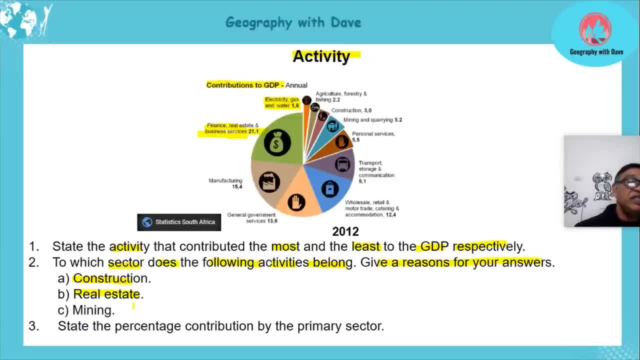 service of selling. okay, that is when you sell it. it's tertiary. and then, lastly, it's mining, where you extracting raw materials from the earth. okay, and that becomes your primary. so, secondary, tertiary, primary, all right. so you now you're asking to classify them. look at the last one state. 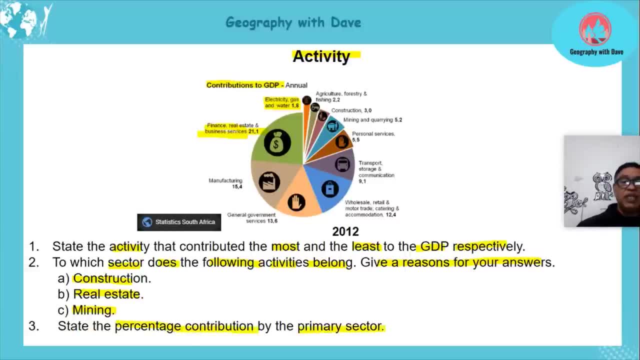 the percentage contribution by the primary sector. now, what do i need to do here? i need to identify which ones is the primary sector. i'm looking here, i see whoa. there's agriculture here 2.2. ah, there's mining here 5.2. so 2.2 plus 5.2 is 7.4. i'm checking, checking. now, these are all secondary. 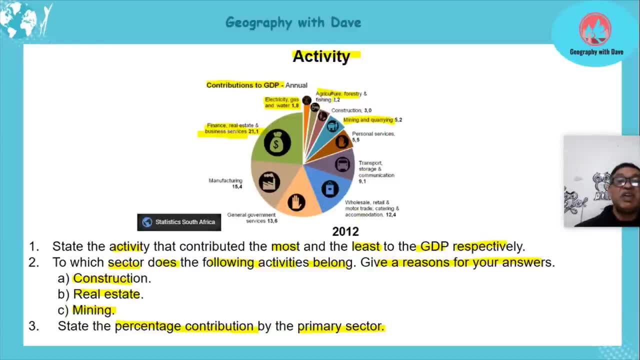 and tertiary. all right, so i got it. and if i look at 2.2 plus 5.2 is 7.4 percent. all right, some just simple things here, but sometimes we find learners- it's a simple things- that you don't get right. that then creates challenges for the so-called more challenging questions.